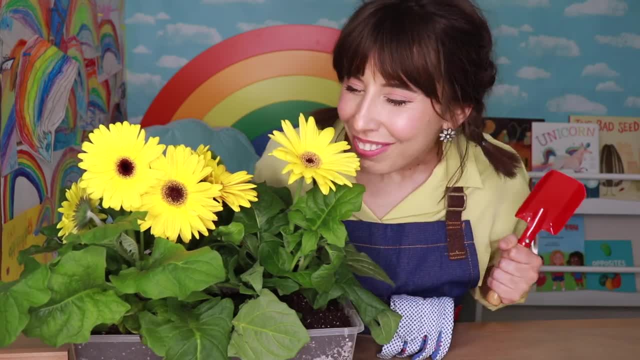 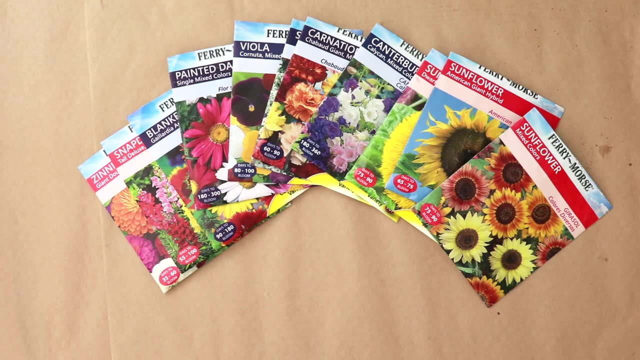 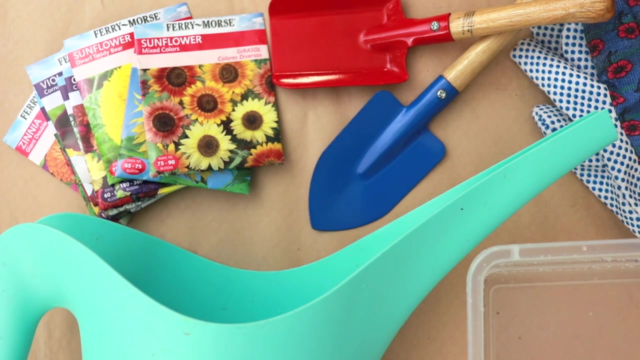 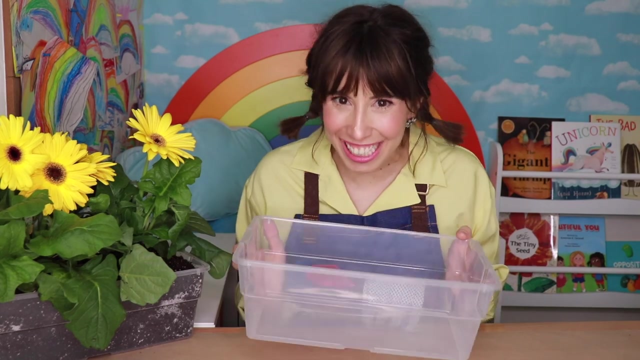 into a beautiful flower. For this project, I'm using seeds, a container for my plant, soil, a watering can and optional gardening tools and gloves. I'm starting with this container. You probably have something at home already that can work as a garden pot. It's okay to be creative with what you find It works best. 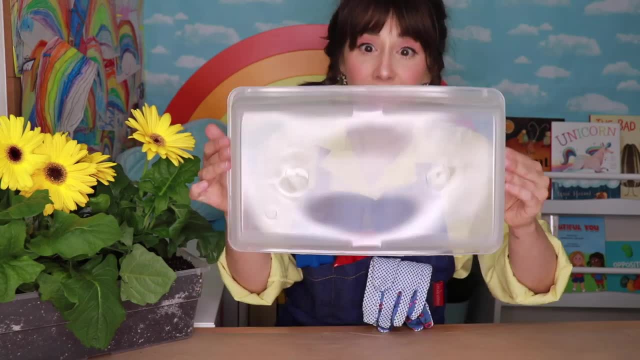 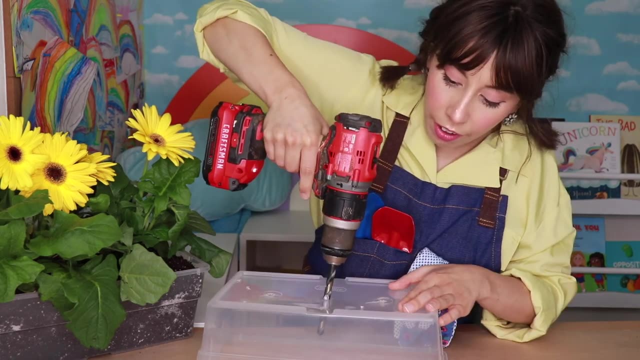 to have holes in the bottom of the pot. I'm going to put a hole in the bottom of the pot. You can even make your own holes with the right tool. If you're trying this at home, ask a grown-up for help. Next, let's add soil. 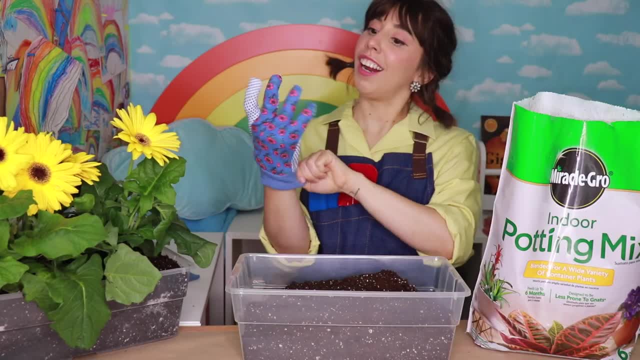 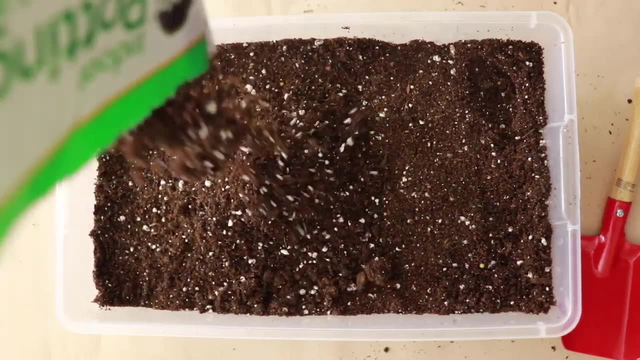 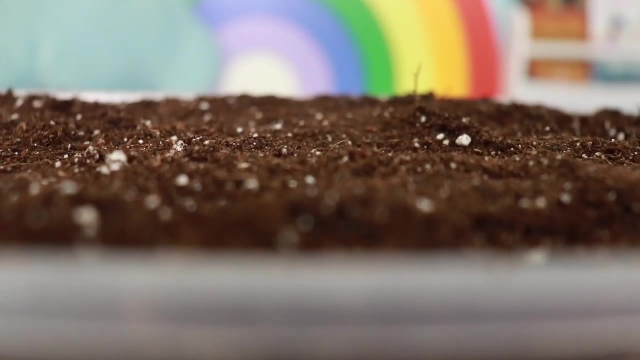 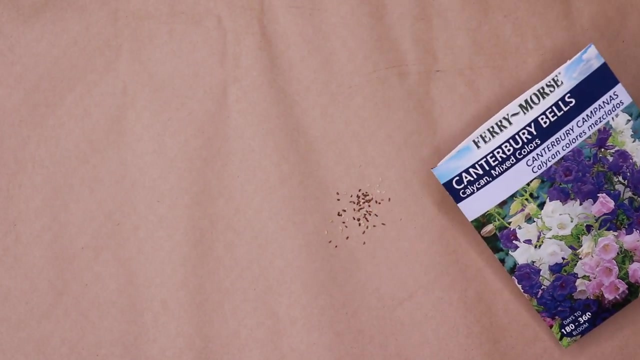 No matter what kind of seeds you have- fruit, vegetables, herbs or flowers- they all need soil to grow. Fill up your container all the way to the top. Now it's time to plant your seeds. Just like the flowers they grow into, seeds come in all kinds. 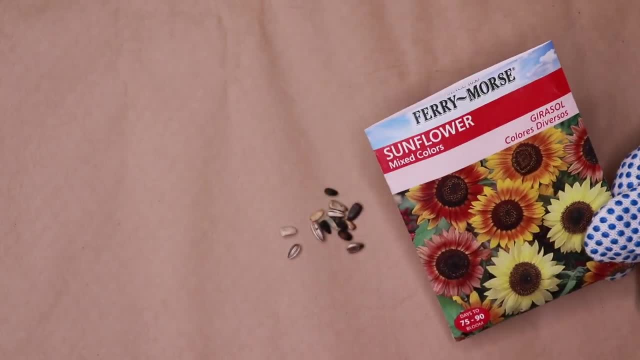 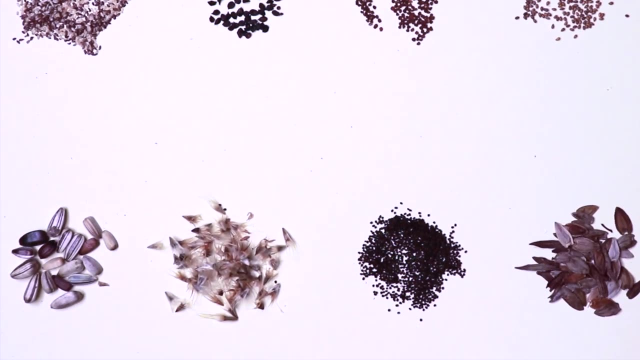 of different shapes, sizes and colors. Just look at how different all of these flower seeds are. Activate the林 leaves on top of the flowers. Let them harvest with one flower of depth that 35 centimeters deep. Plant a first flower and Next. 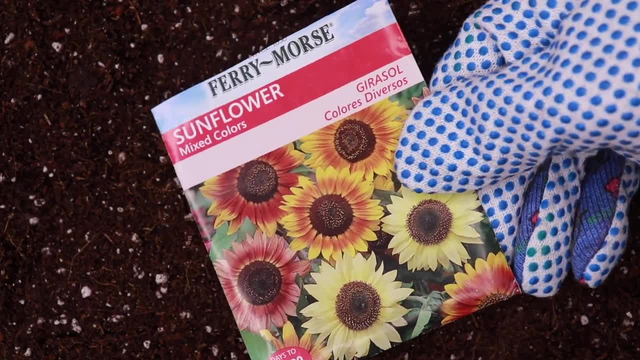 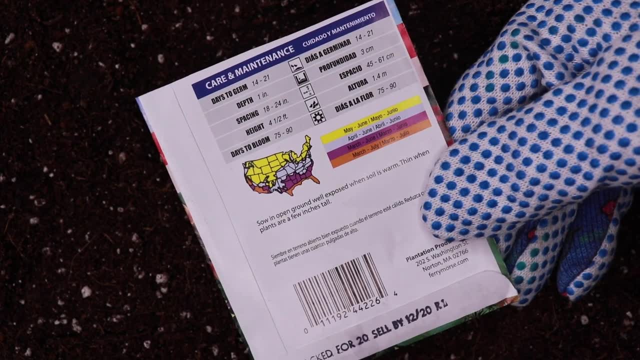 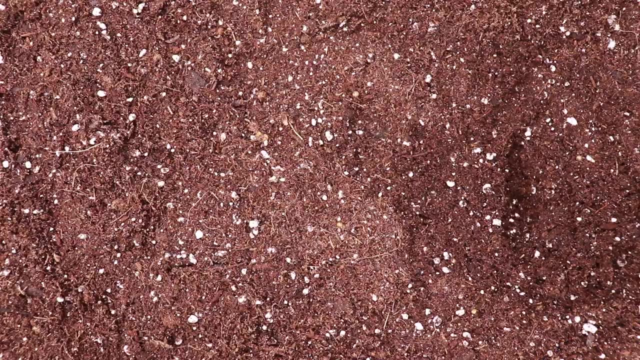 ffe, next flower and Next mini sunflower seeds. the back of your seed packet will have lots of important information, like how deep to plant your seed. mine said one inch. i checked on a ruler and used my shovel to dig a little hole, drop in the seed and cover it up again. 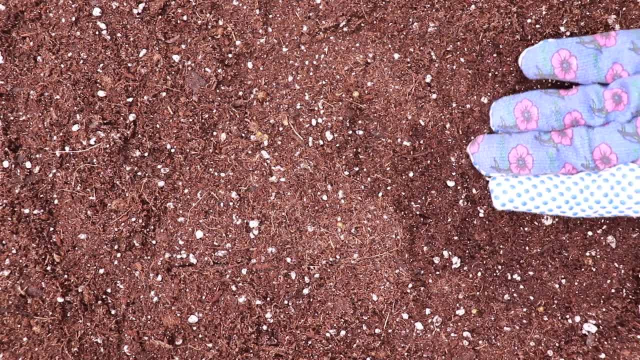 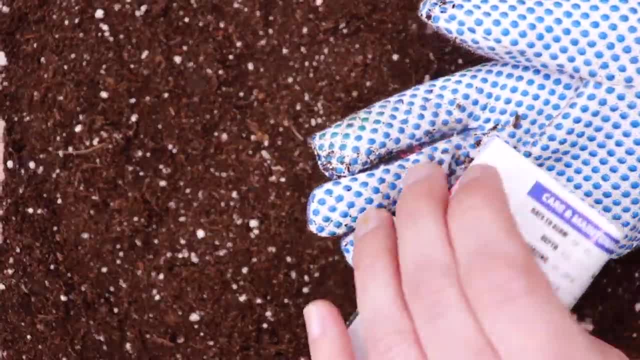 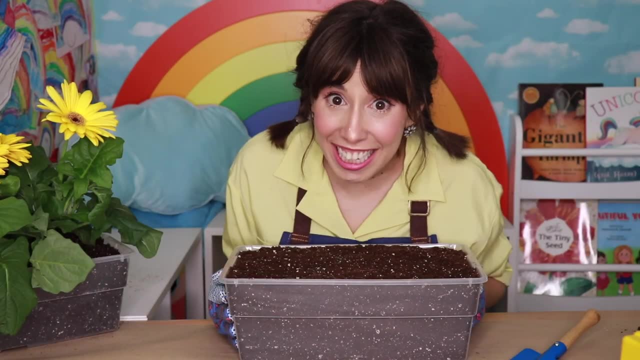 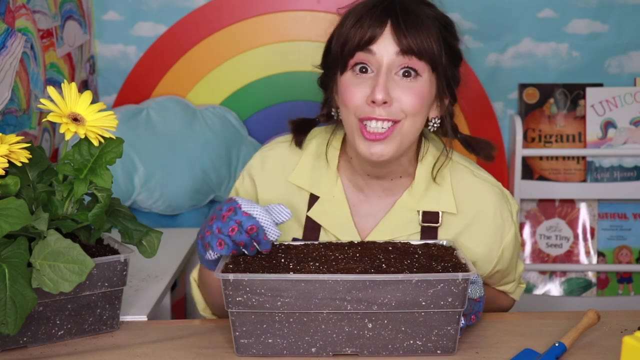 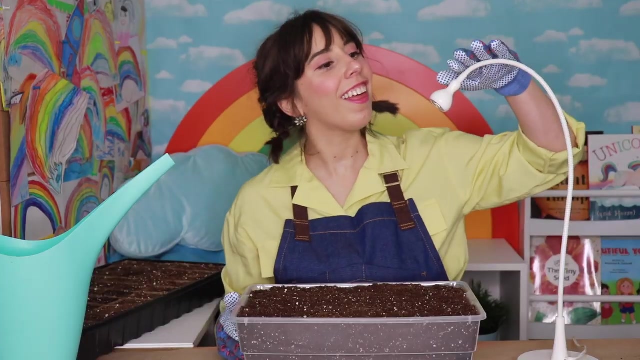 you can also use your finger to make a hole and cover it back up now that our seeds are in their new home, buried, nice and cozy in the soil. they need two things to grow: water and sunlight. so plants do best in natural sunlight. if you don't have an outdoor space where you live, 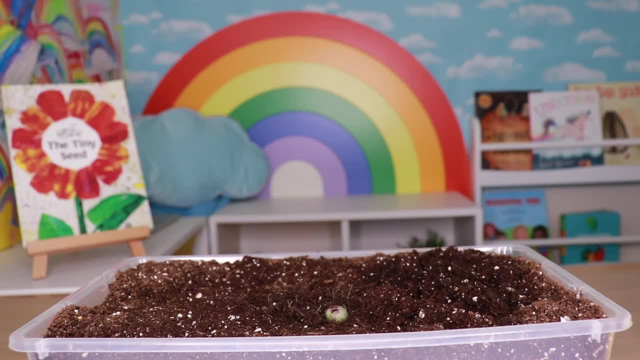 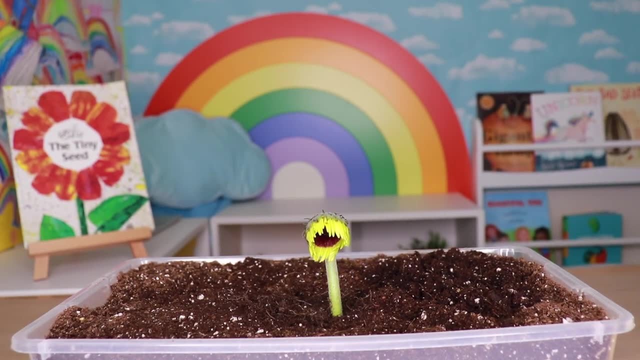 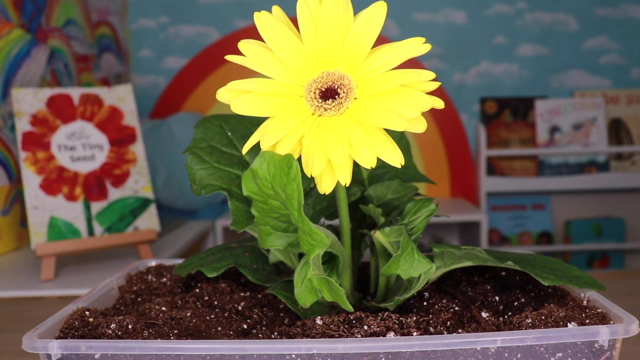 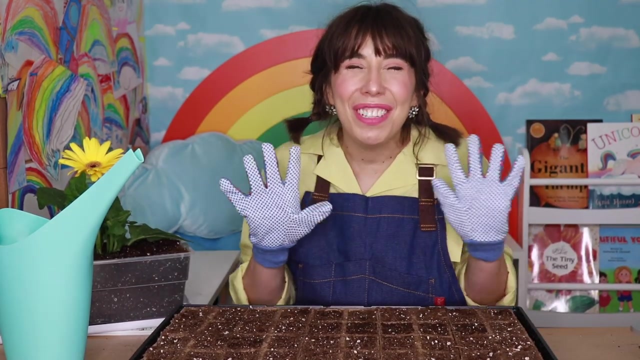 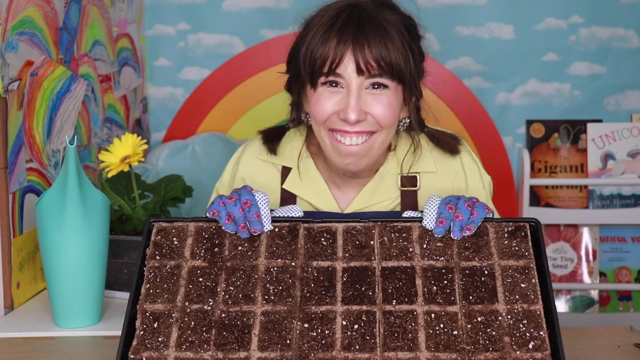 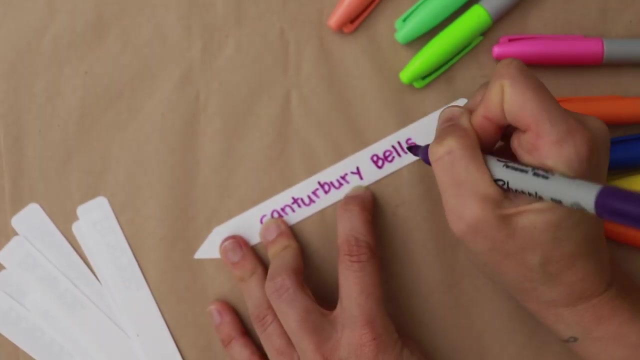 you can use an indoor light. over time, your seed will shed its shell, sprout and little by little grow into a big, strong plant. i decided to plant many more different seeds. i hope to grow a colorful flower garden. what's your favorite kind of flower? oh, you can label your plants with a popsicle stick or something similar, so you don't forget. 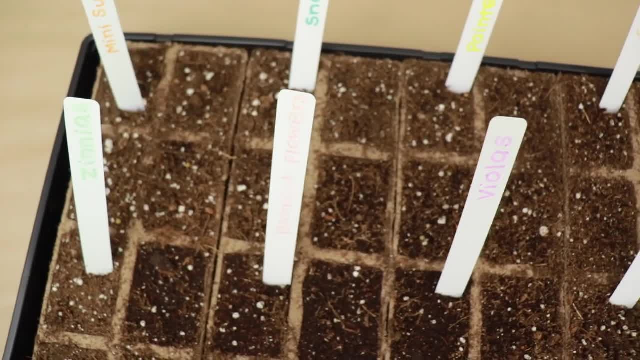 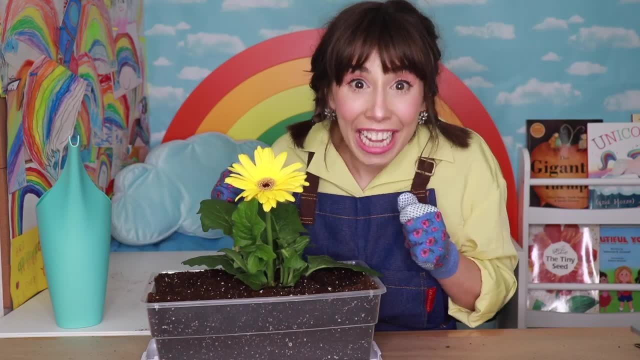 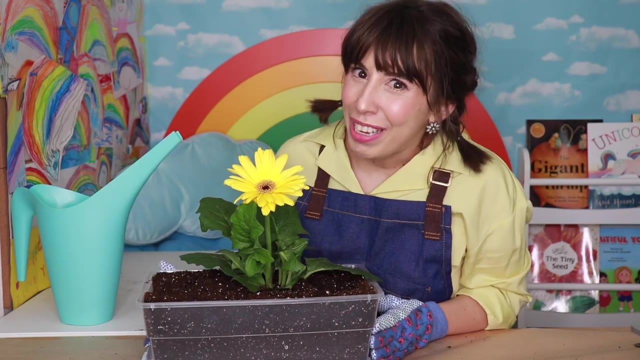 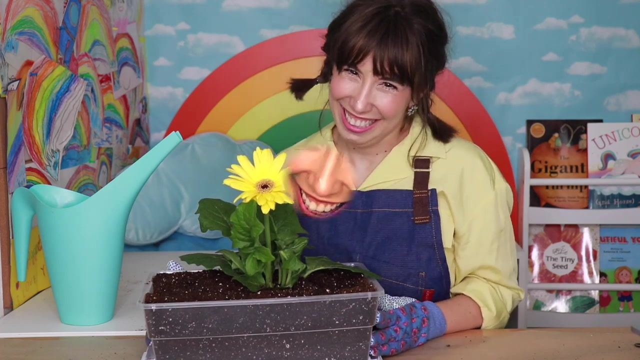 what kind it is. that was lots of fun. the seed was growing, the seed kept going. i hope you enjoyed this video and i'll see you in the next one. bye, bye, bye, bye, bye, the tiny seed. hey, will you sing a song with me? let's sing about the tiny seed. 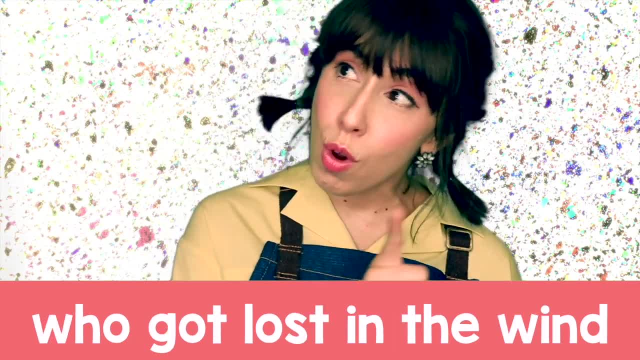 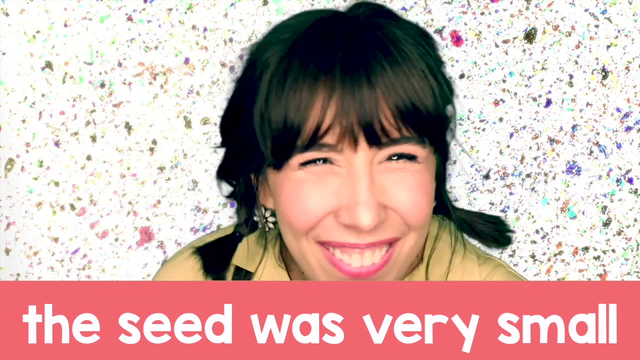 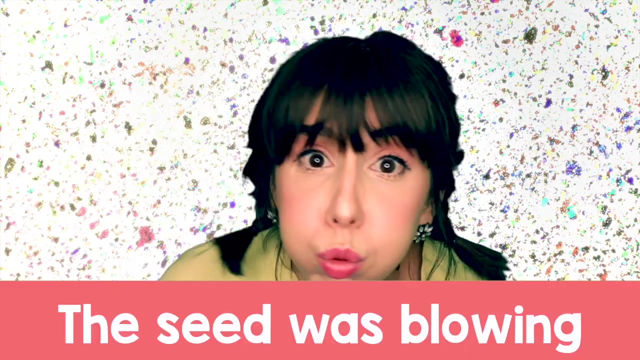 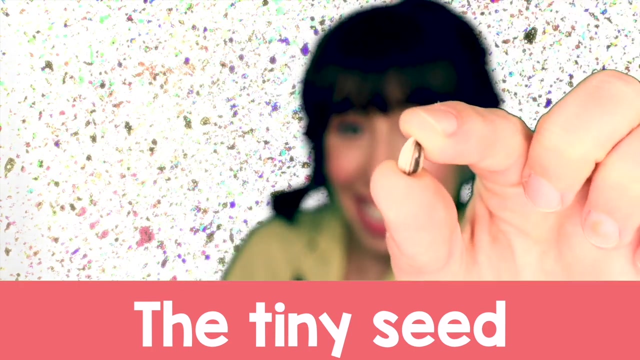 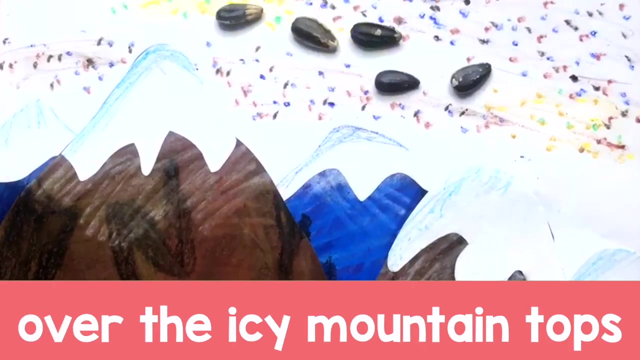 once there was a seed who got lost in the wind. the seed was very small, much smaller than its friends. the seed was very small, much smaller than its friends. The seed was blowing. the seed kept going- the tiny seed- Higher and higher toward the sun, over the icy mountain tops. 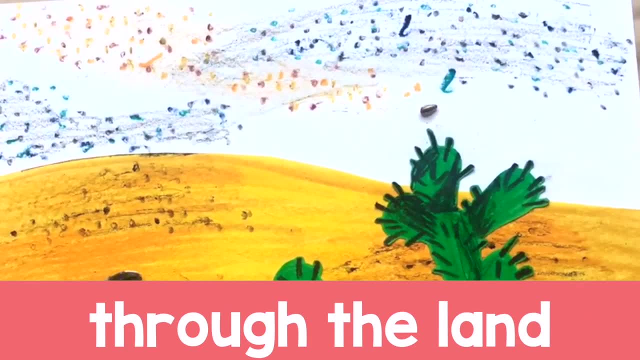 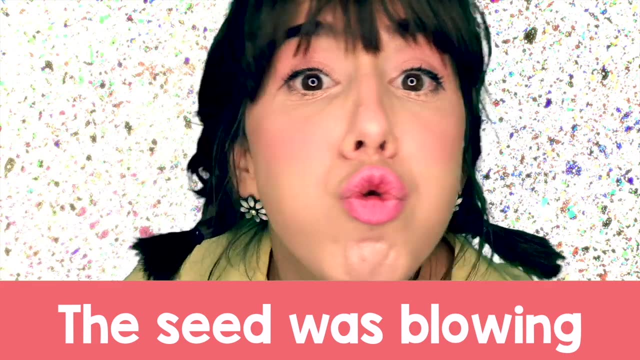 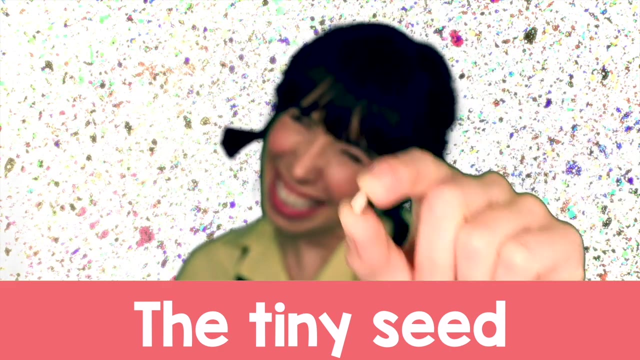 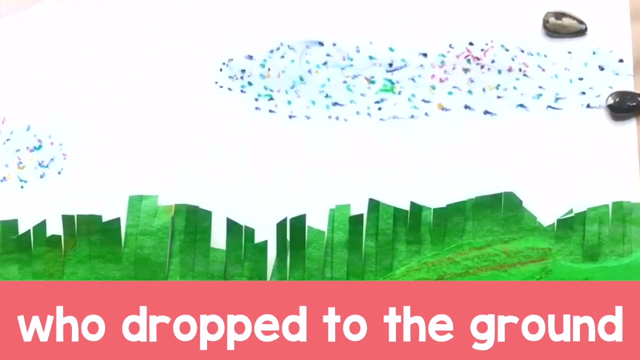 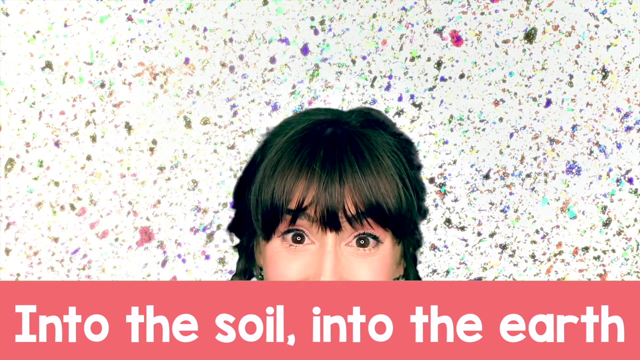 Across the great ocean, through the land, over the farmer's crops. The seed was blowing, the seed kept going, the tiny seed. Once there was a seed who dropped to the ground, Into the soil, into the earth. its home had been found. The wind stopped blowing, the seed kept going, the tiny seed. 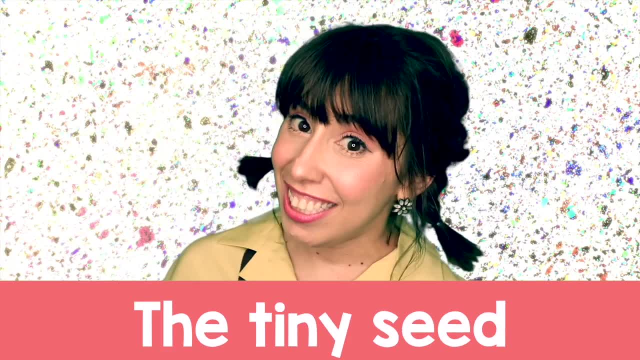 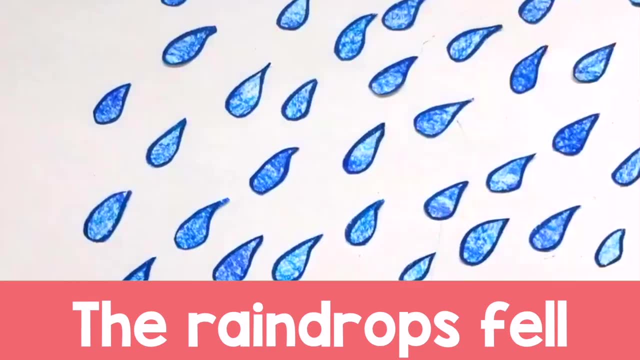 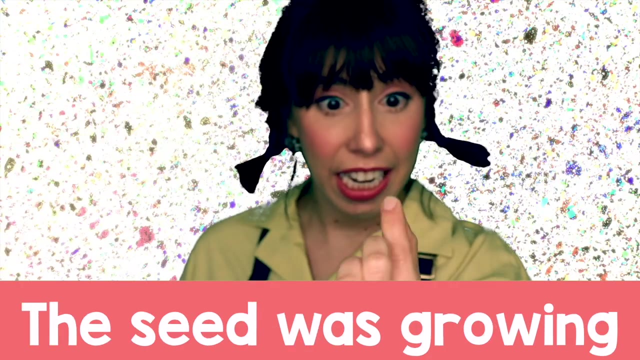 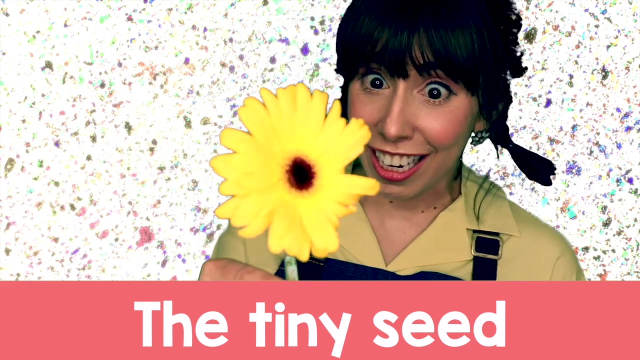 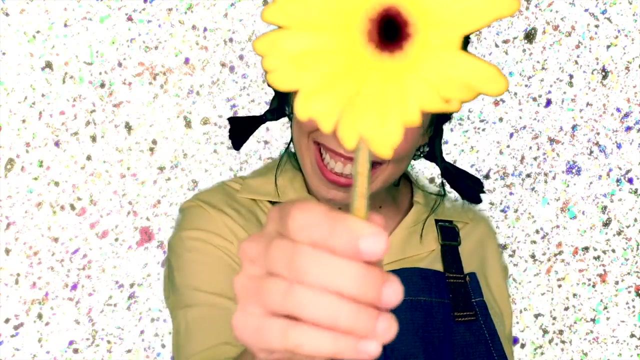 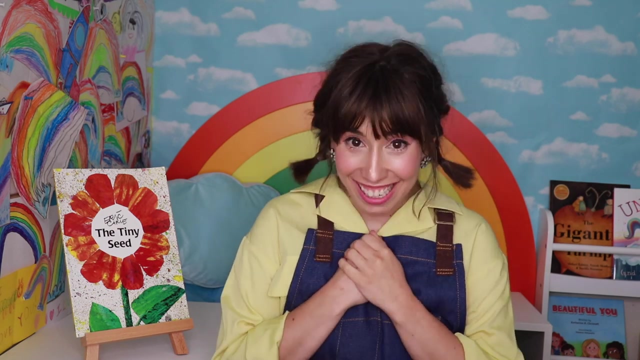 The sun shone bright, the raindrops fell, The seed burst out and shed its shell. The seed was growing, the seed kept going, the tiny seed, Higher and higher toward the sun, over the icy mountain tops. Thank you for singing with me. Flowers are so beautiful. 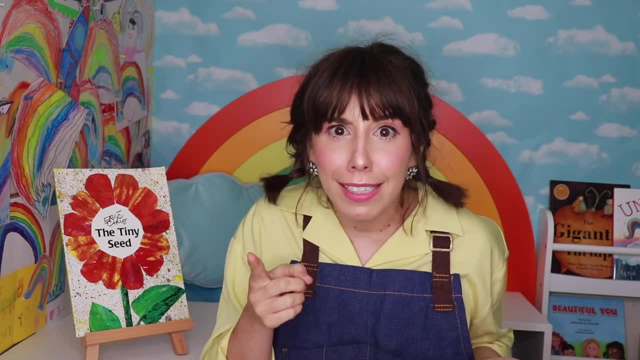 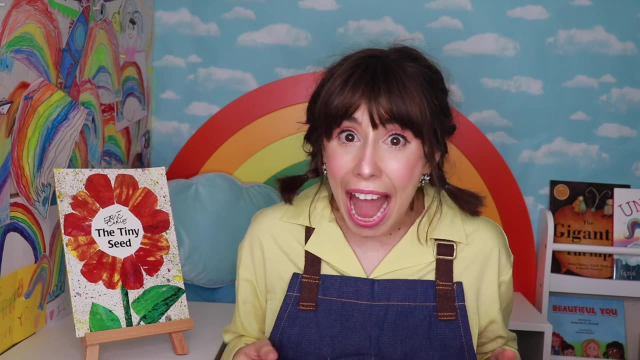 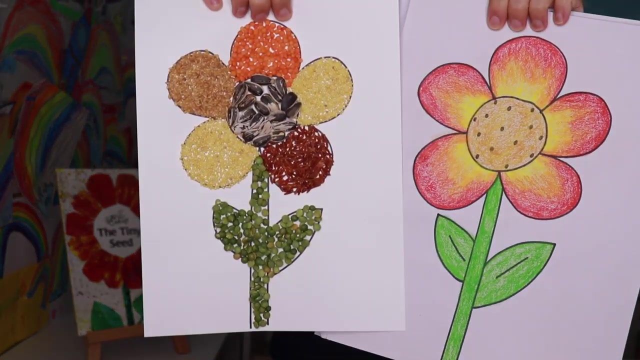 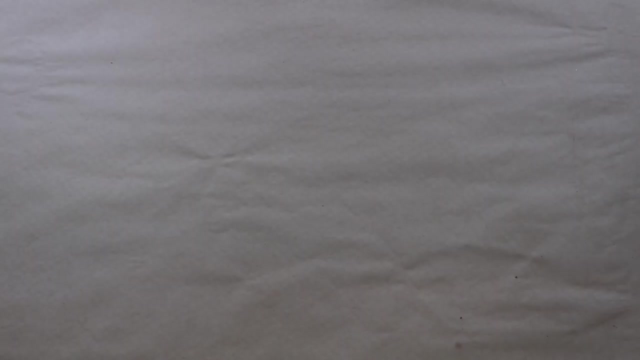 They come in all kinds of different shapes, sizes, smells, colors and patterns. Today, let's draw and design our own flowers Like this. First, I'll show you how to make the mosaic flower. You'll need paper, a black pen or marker to outline. 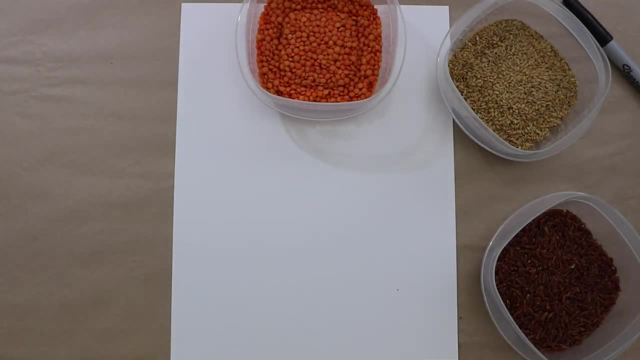 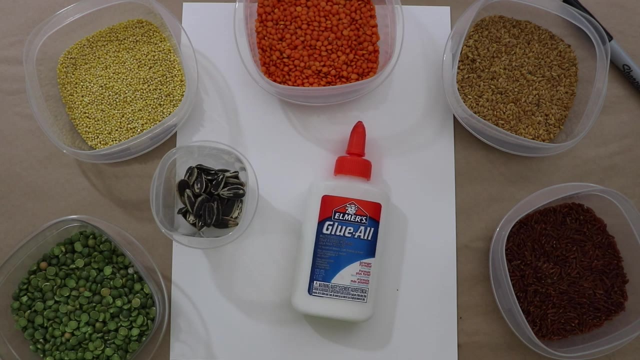 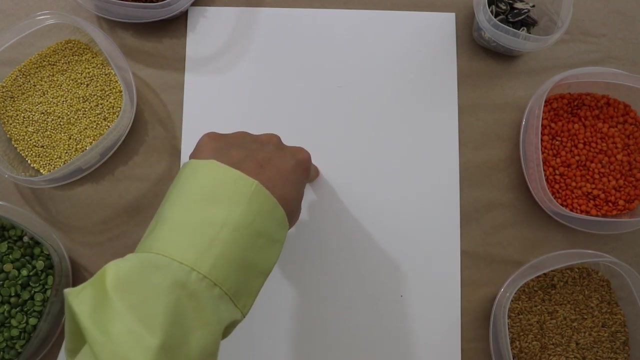 and next seeds, rice, lentils, beans, any kind of dry food you can find- Different colors are great. And last, glue With your outlining marker let's draw the flower, Find the center of your page and jump up a little. 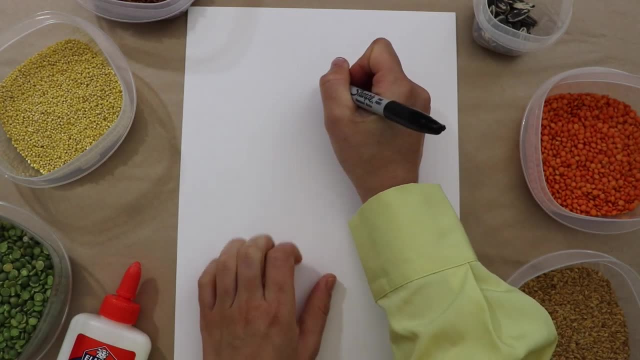 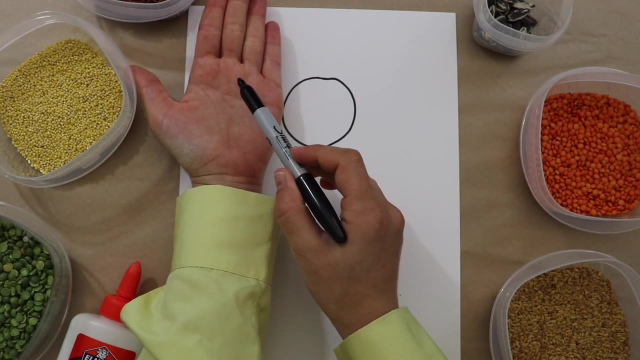 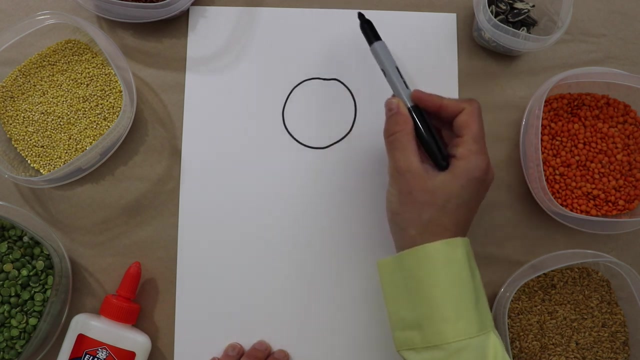 Here's where we'll make our center circle for the flower. When you draw the circle, try to keep it small enough to fit inside your hand. Next, we'll draw the petals of the flower. We'll try to make them all about the same size. 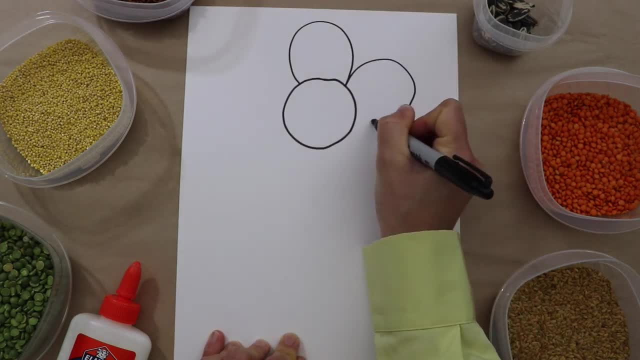 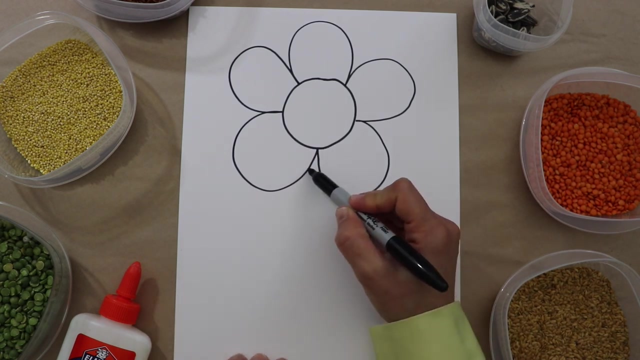 I'll start here and go around Boing, boing, boing, boing and finish at the same spot I started. Next, the stem. Use your finger to see how big the stem should be. Now some leaves. 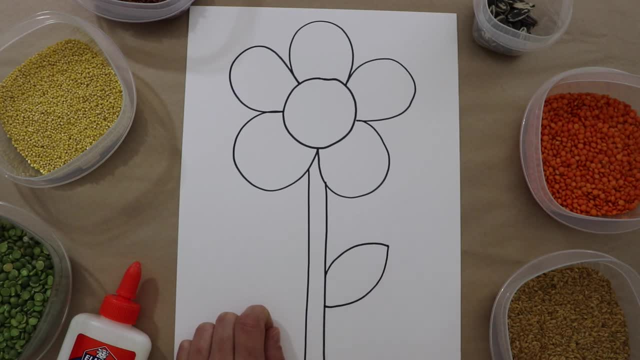 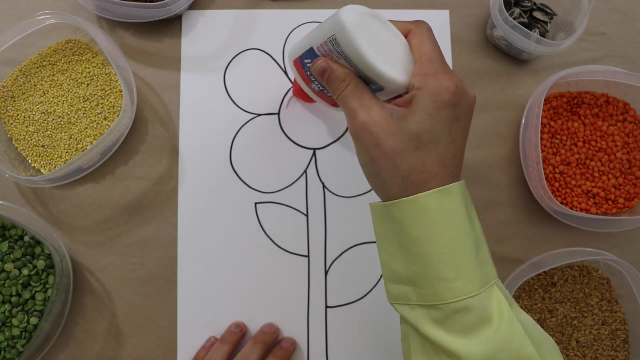 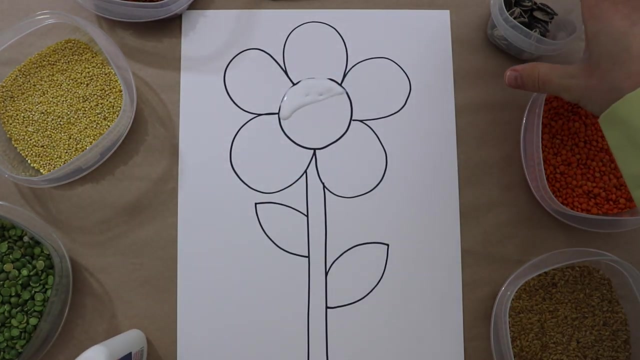 Go out and back And on this side, Go out and back. Great, Now it's time to glue on our seeds and dry foods. I'm starting with the middle circle. I'll start with a small section. first, Don't squeeze the glue too hard. 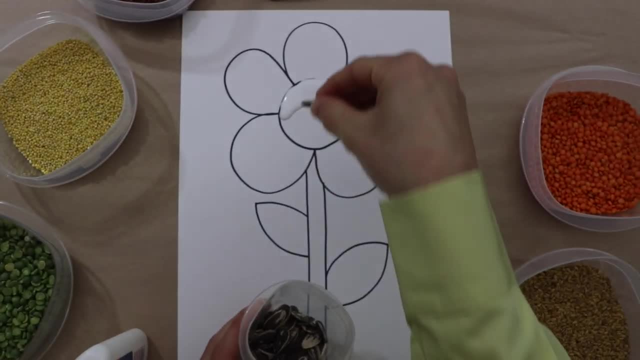 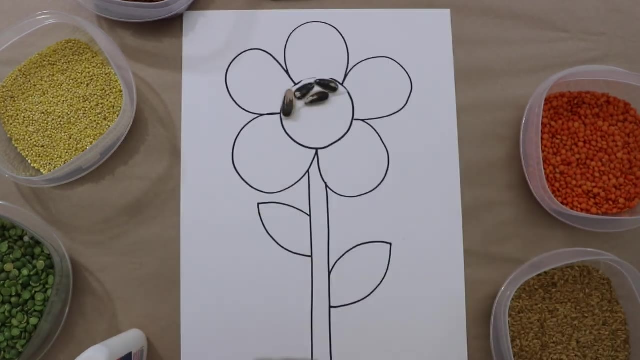 A little bit goes a long way. Drop your seeds. Do the same with the other side of the flower. Drop your seeds in the glue and push down lightly. Then keep going. A little bit more glue, A little bit more seeds. 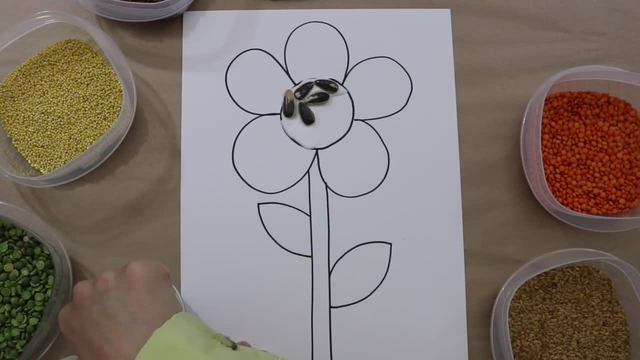 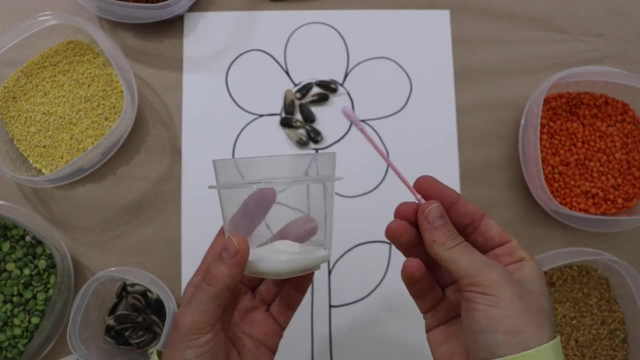 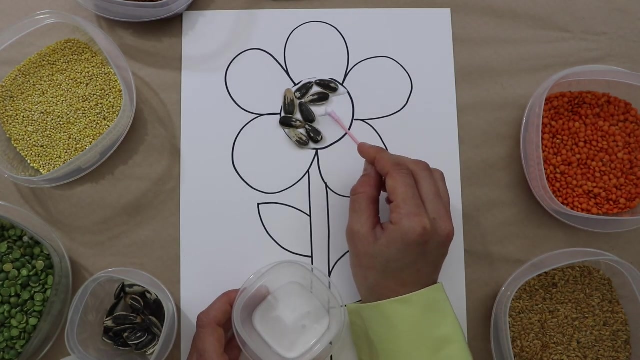 I'm using sunflower seeds for the center of my flower. It helps to use a Q-tip to dip in the glue so you don't use too much at once. You may want to use a small tip for this step. You can use a little bit at a time. 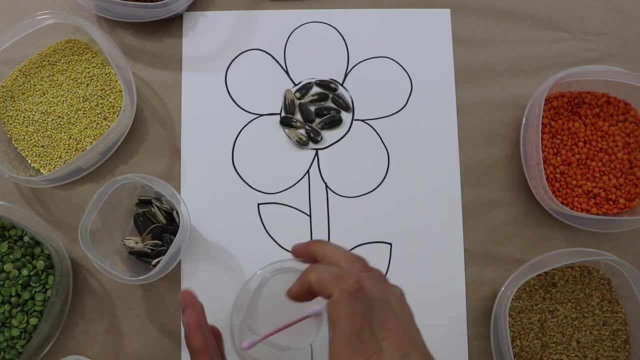 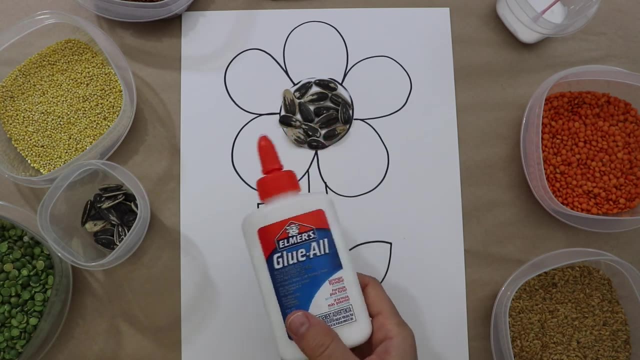 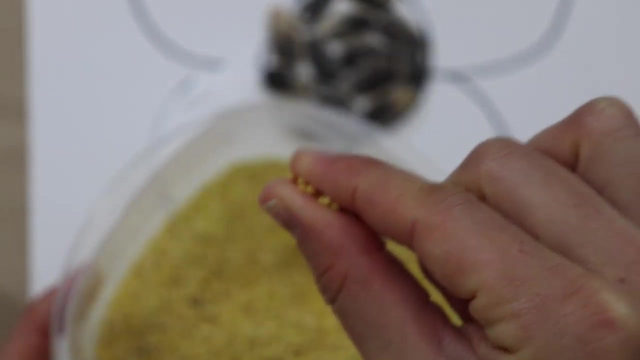 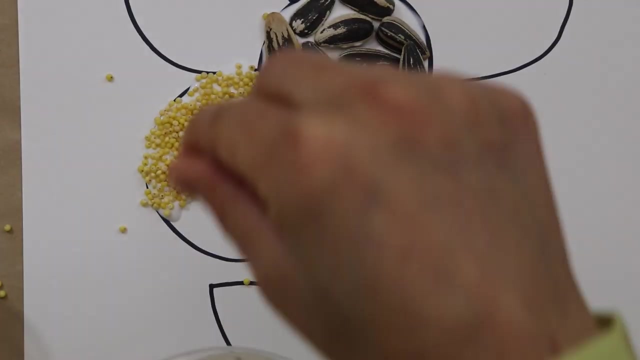 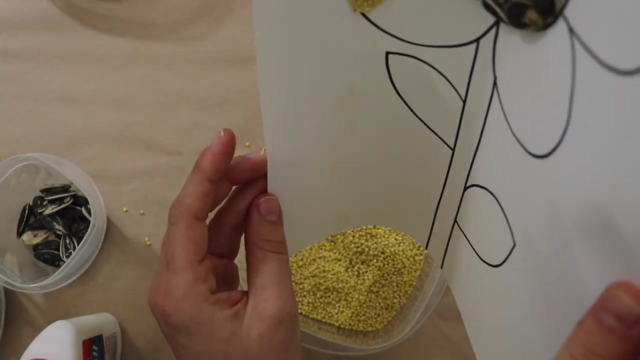 You may also want to use a little bit more Now. one by one, we'll fill in the petals. Take your dry food and pinch just a little. Drop it on the glue Slowly and carefully. it can get pretty messy. I just pour the extra back into the jar. 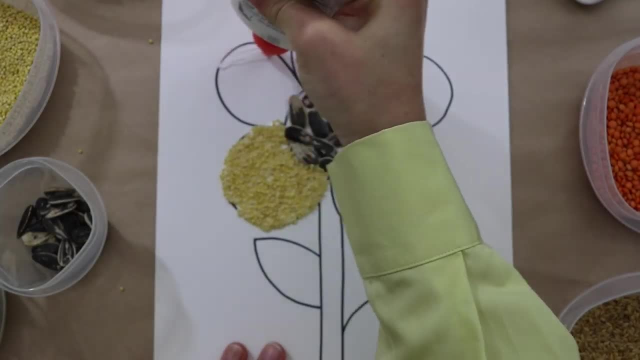 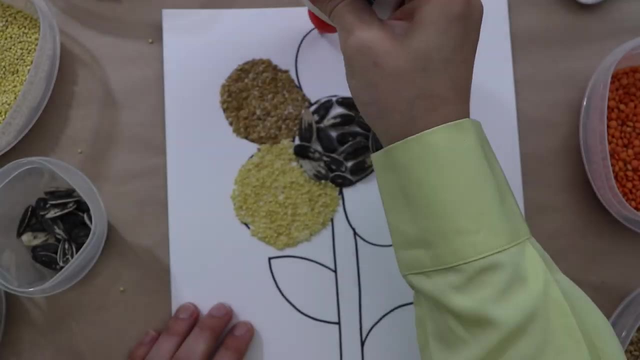 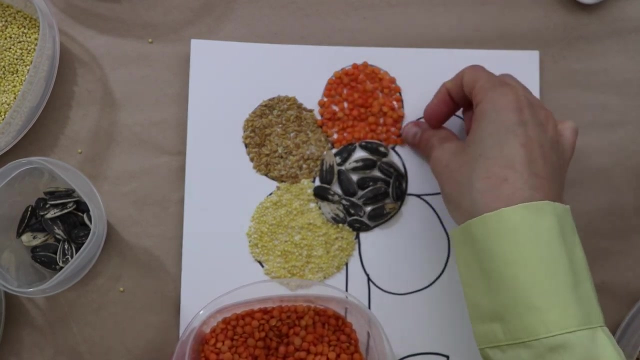 Keep going. Little bit of glue, little bit of food. Little bit of glue, little bit of food. I'm using golden flax seeds for this petal, And this one is red lentils. yummy, I'll use the same quinoa I used before. 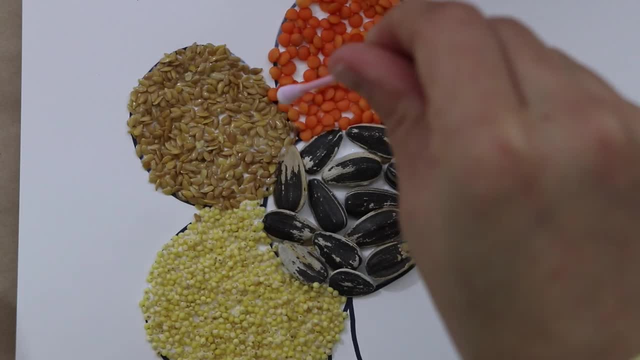 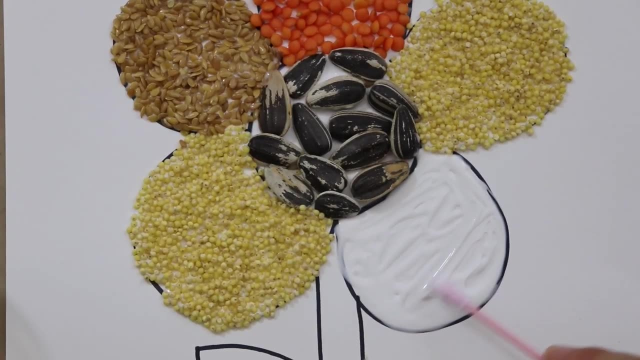 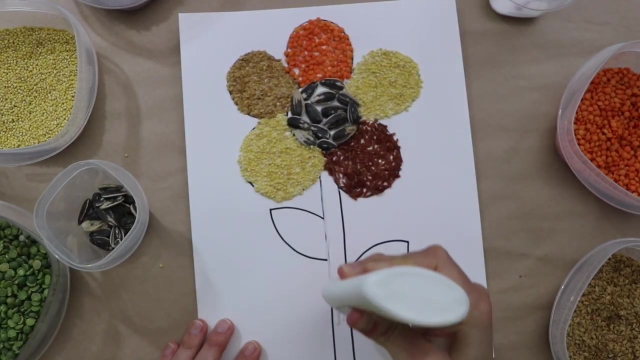 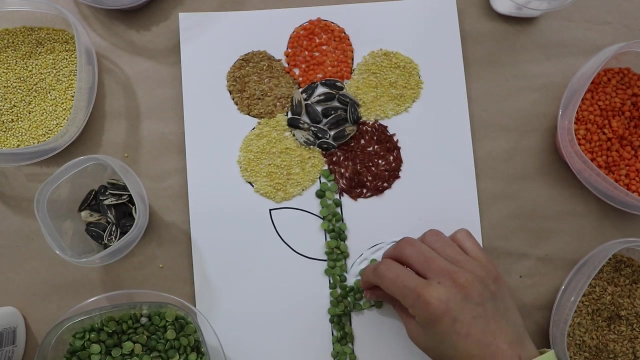 Because I like yellow and this food is a yellow color. Remember, you can always go back and fill in some holes or pieces that fall down. I've got some red rice for this petal And last I'll use split green peas for the stem and leaves. 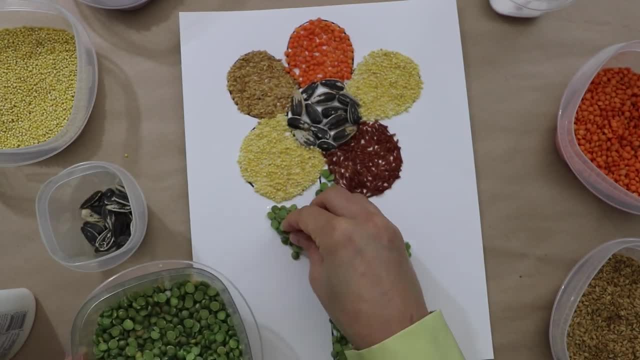 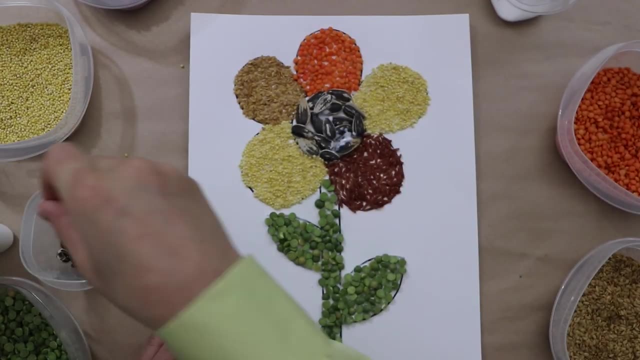 Little bit of glue, little bit of food. Little bit of glue, little bit of food. There, I'm gonna fill the petal with a little bit of yellow food. I'll just fill in some last pieces. Tada, Maybe you just feel like coloring. 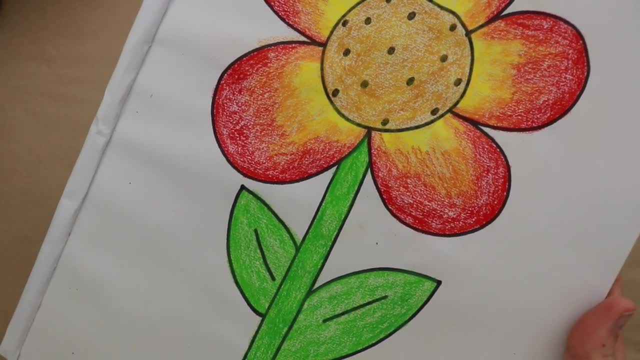 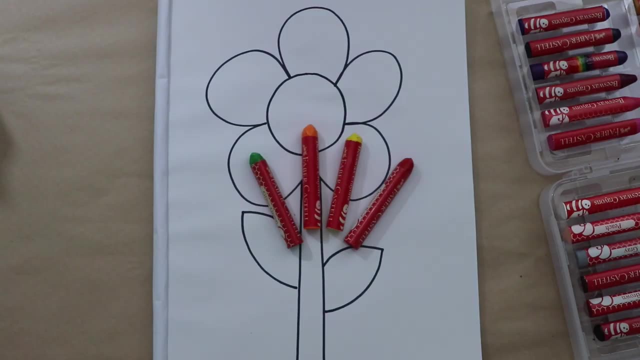 Well, I'll show how I like to color in this flower. Start with the same outline we used before. This time you'll need something to color with. I'm using crayons. I'll take my same outlining pen and draw some dots. 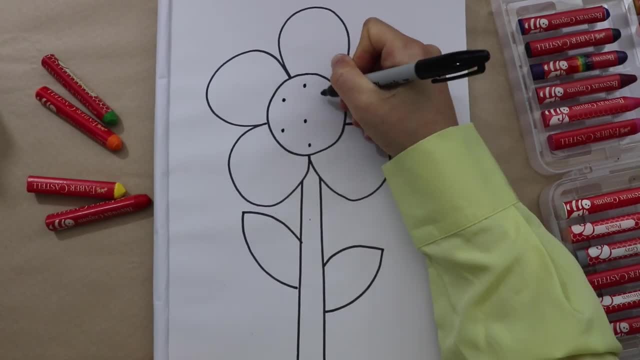 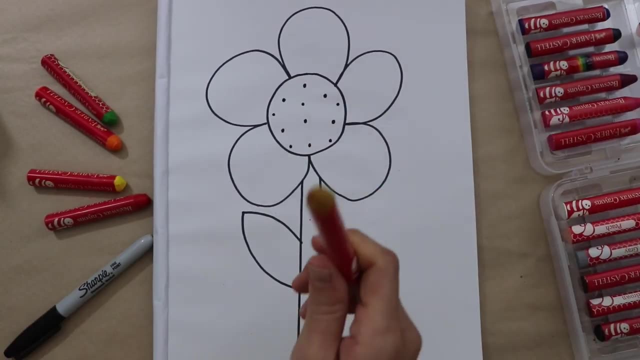 Perfect, I know I love it. Talk about cool. Bye, bye, Bye, bye, I love it. Happy new year. Bye, bye. This represents the seeds that live in the middle of the flower. Now I'll use a color for the middle of the flower. 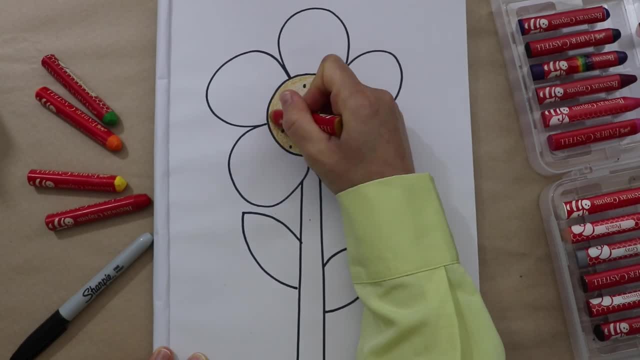 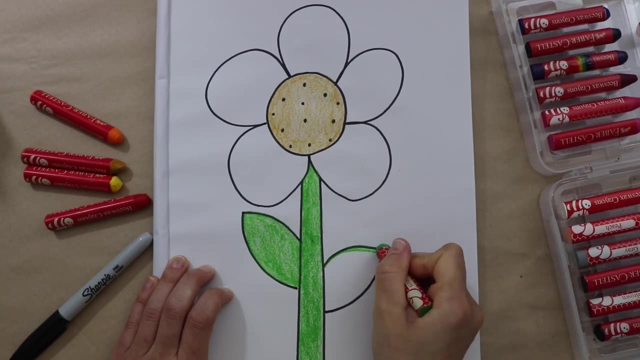 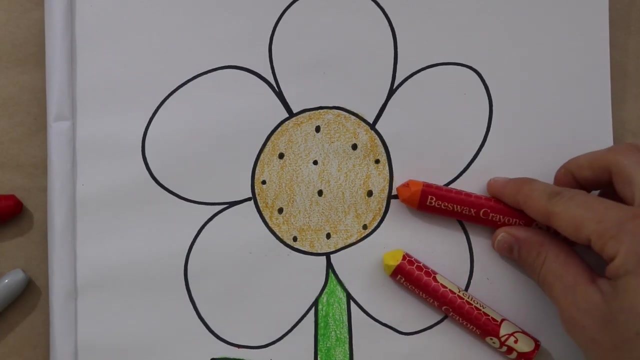 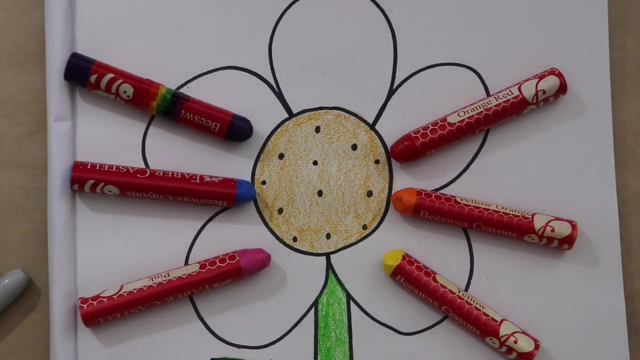 I chose a golden yellow color. Next I'm using green for the stem and leaves. Now you can choose three colors for your flower: Something light, medium and darker. It could be any three colors you like. Today I'm starting with yellow. 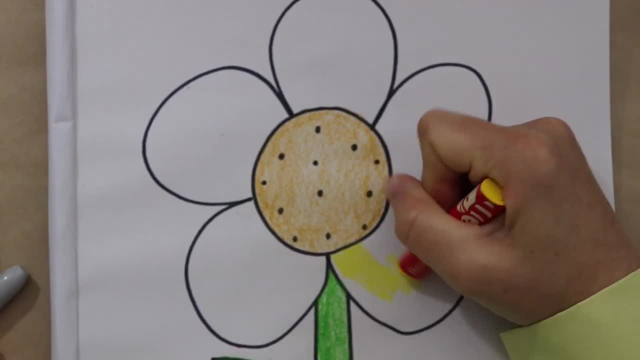 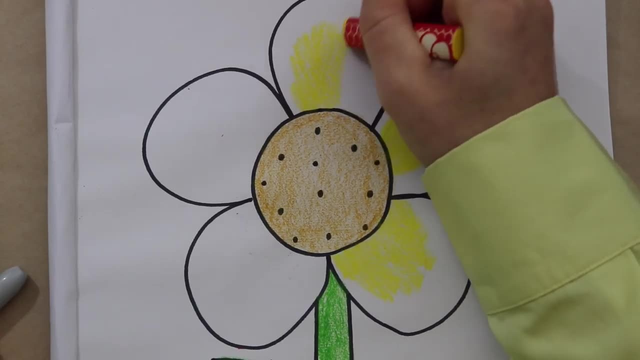 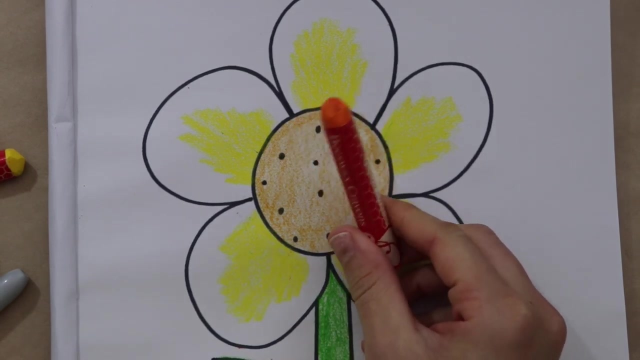 Inside the petal. you're going to color, but not all the way to the top, Just about halfway. Keep the same shape as the petal with a rounded top like this. Take your second color and start to color. Start to color on top. 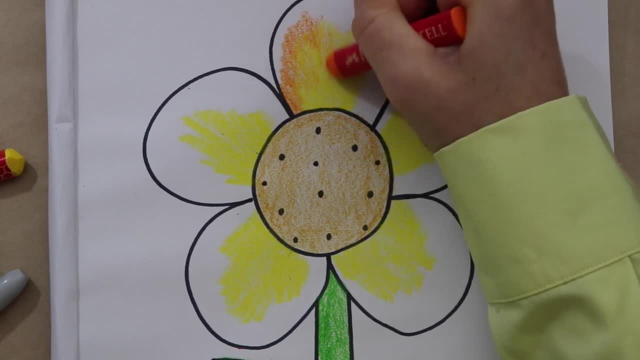 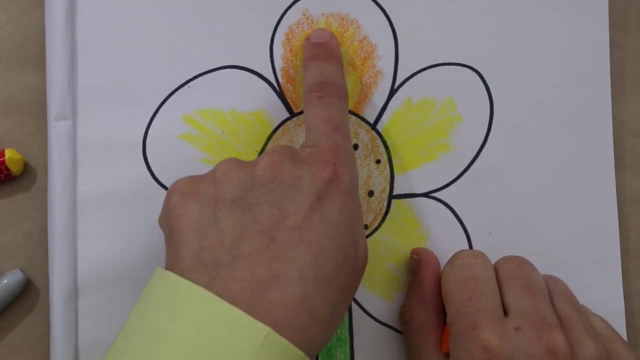 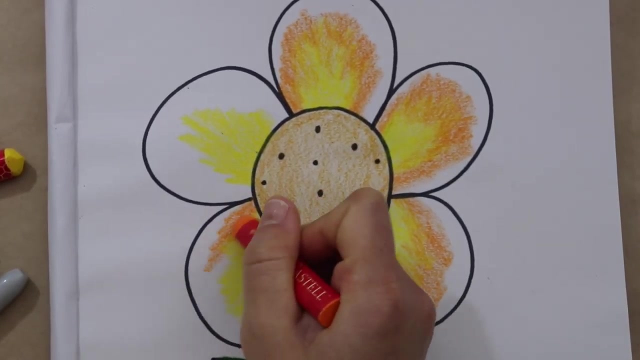 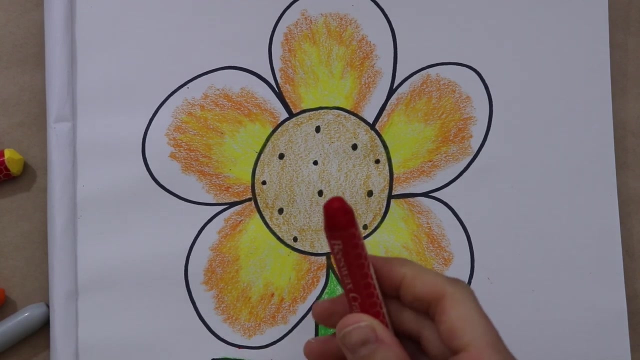 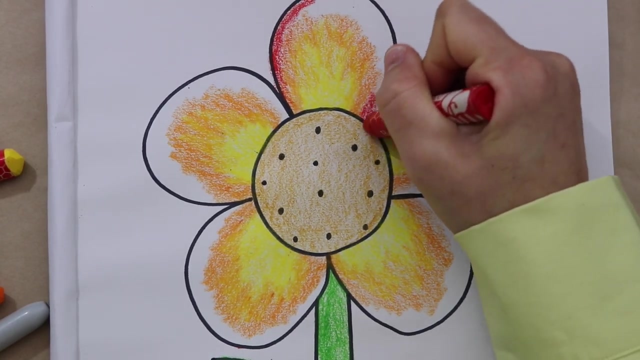 Go over the yellow or the color underneath just a little. We're creating different layers so it looks almost like a sunset. Don't push too hard on top of the bottom color. Keep it nice and gentle. And for our last color, this goes on the outside where you've left some white space. 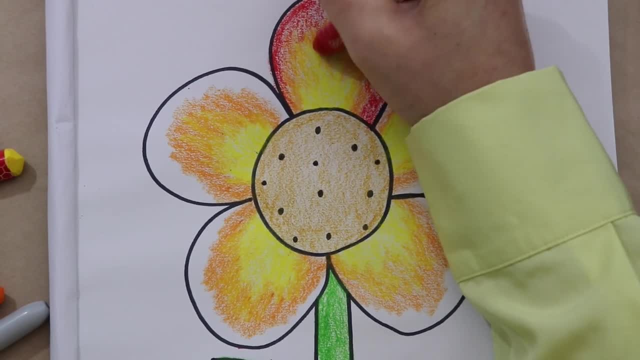 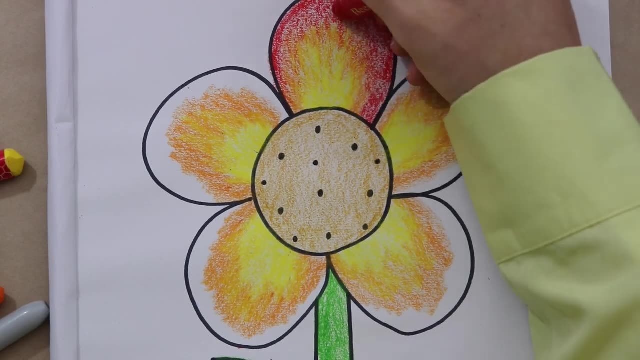 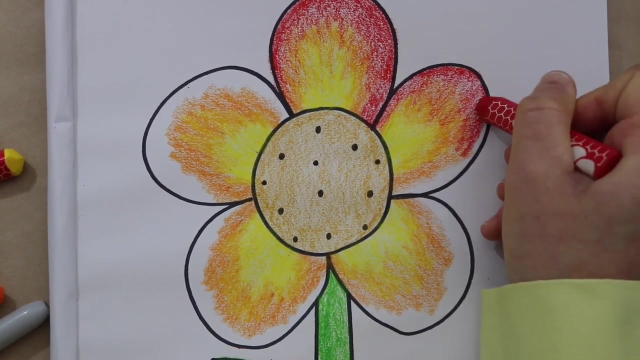 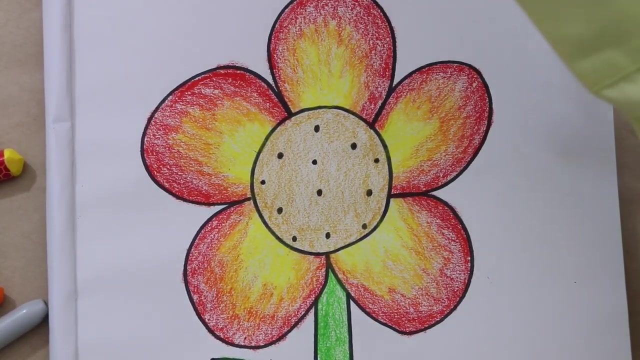 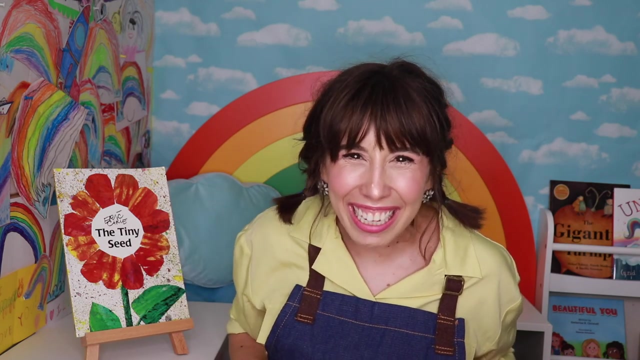 Color it in And again go over your other two colors just a little bit so they all blend together. Repeat for every petal till your flower is all filled in Beautiful. Thank you for drawing and creating with me. Whether you made a mosaic like this,